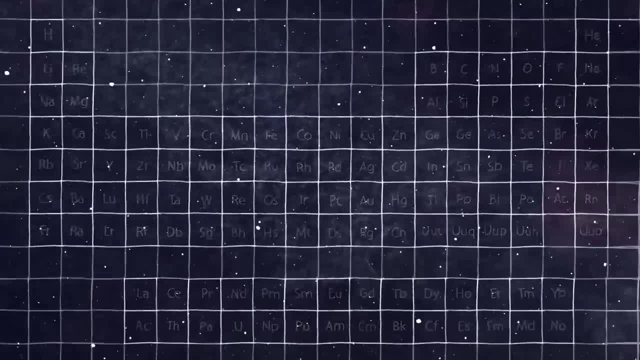 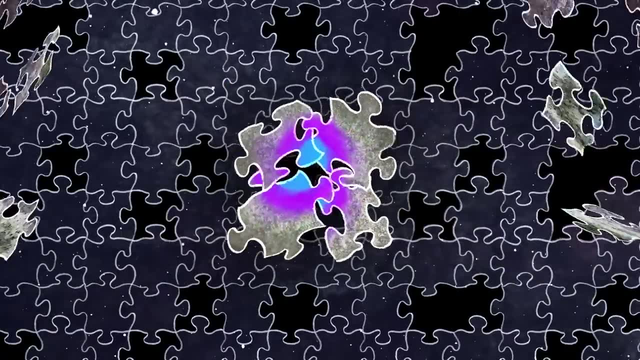 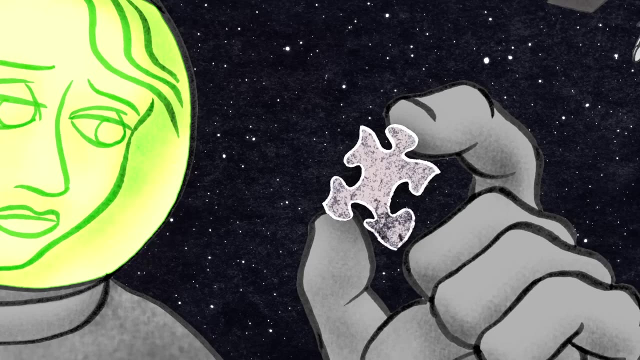 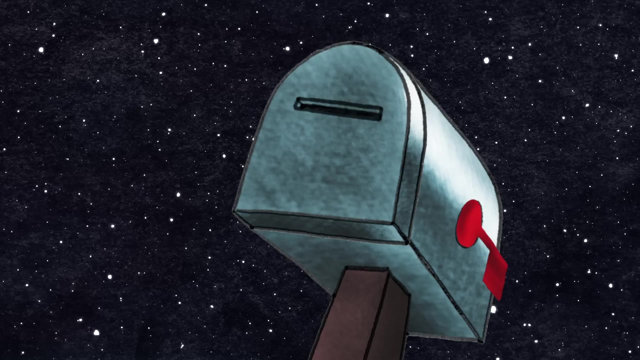 Which elements are the most abundant? Does space contain undiscovered forms of matter? Could there be anti-matter stars or galaxies? Some of these questions cannot be answered solely from visual images, but what if we had messengers bringing us physical data from distant parts of the cosmos, beyond the reach of explorers or satellites? 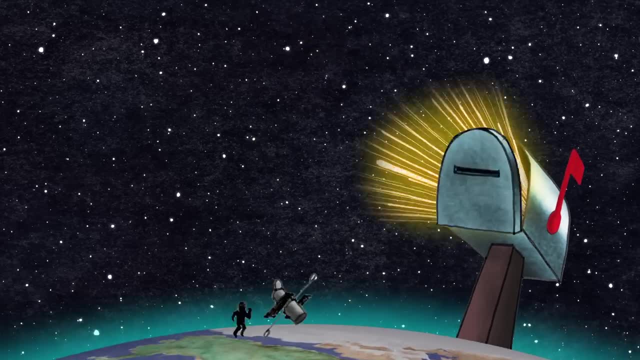 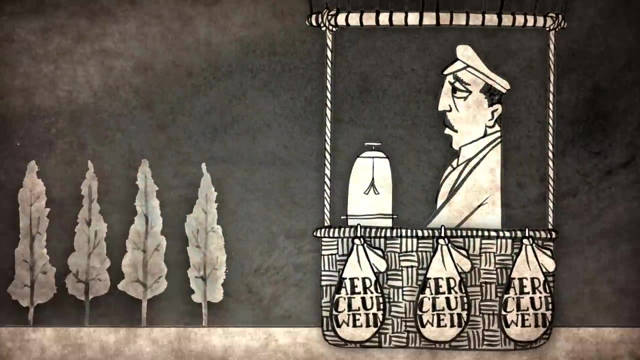 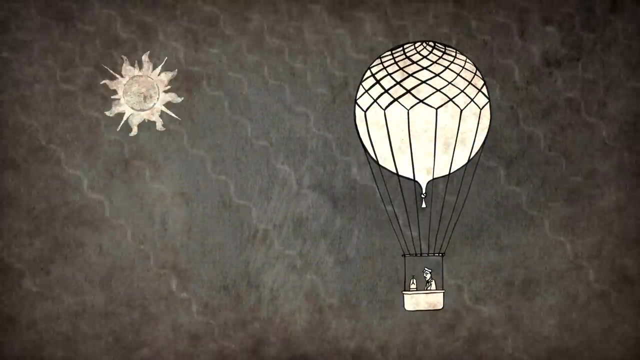 In a way we do, and these space messengers are called cosmic rays. Cosmic rays were first discovered in 1920 by Victor Hess, when he set out to explore variations in the atmosphere's level of radiation which had been thought to emanate from the Earth's crust. 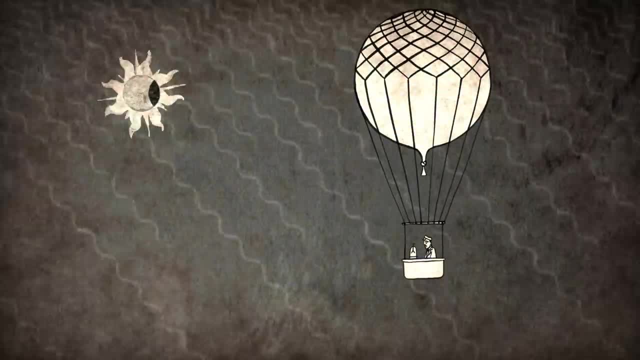 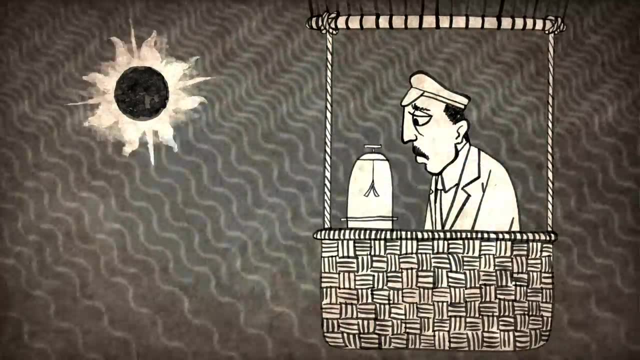 By taking measurements on board a flying balloon during an eclipse, Hess demonstrated both that the radiation actually increased at greater altitudes and that the sun could not be its source. The startling conclusion was that it wasn't coming from anywhere within the Earth's atmosphere. 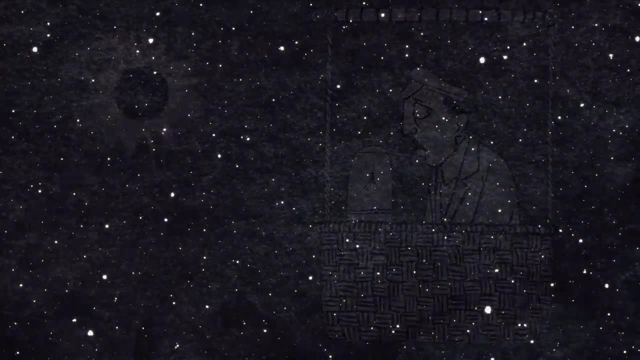 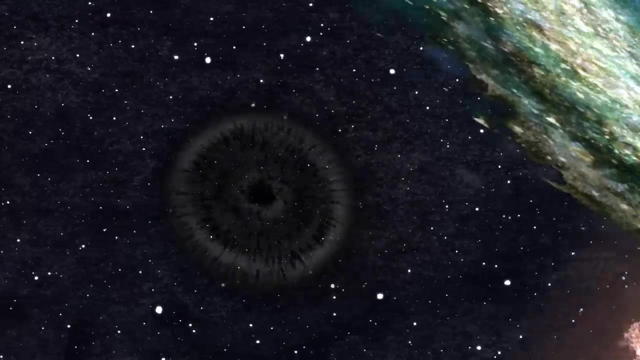 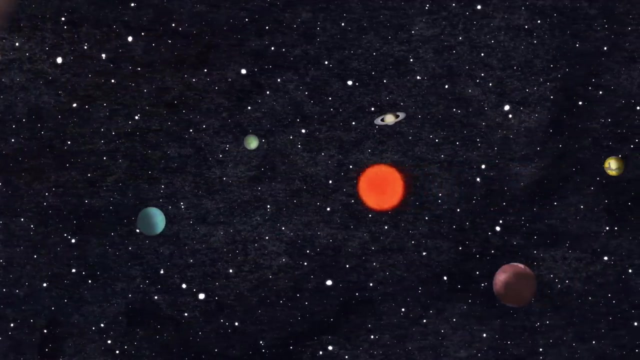 but from outer space. Our universe is composed of many astronomical objects: Billions of stars of all sizes, black holes, active galactic nuclei, asteroids, planets and more. During violent disturbances such as a large star exploding into a supernova. 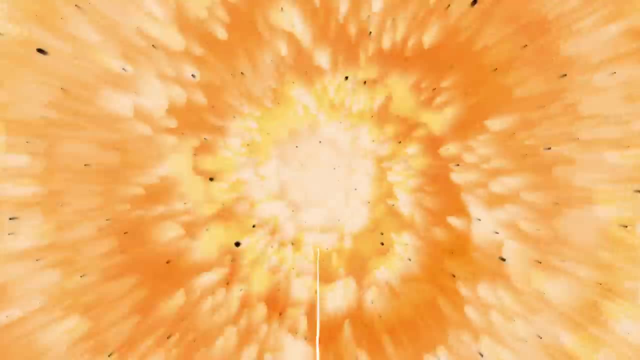 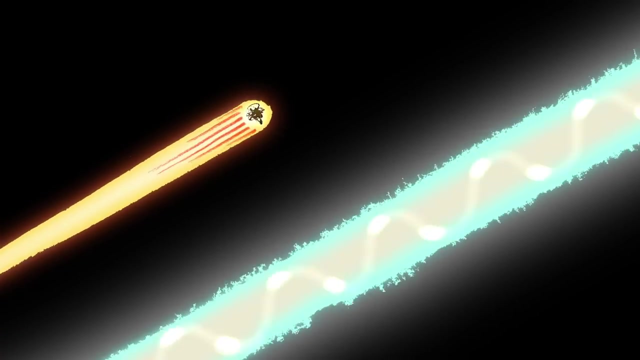 billions of particles are emitted into space. Although they are called rays, cosmic rays consist of these high-energy particles rather than the photons that make up light rays. While the light rays are called rays, they are not the same as the light rays. A light from an explosion travels in a straight line. 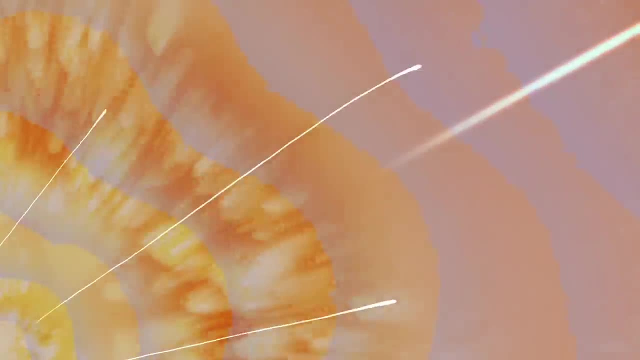 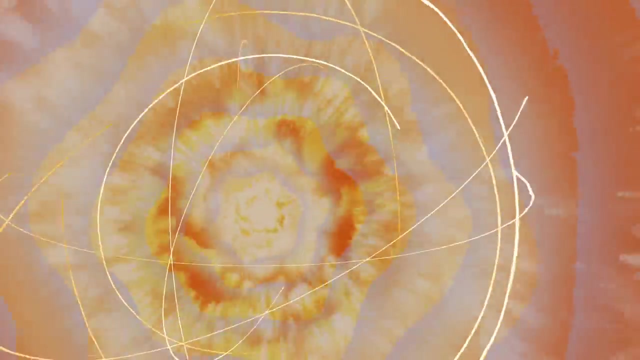 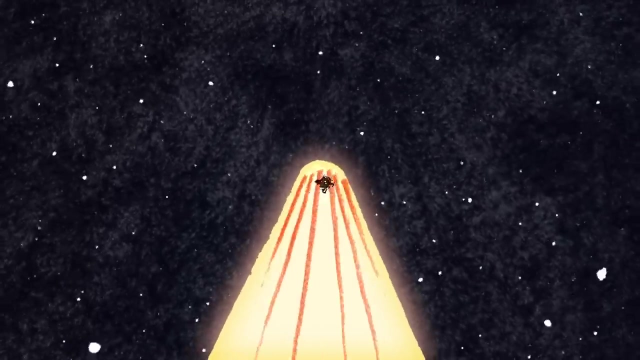 at its famous constant speed. The particles are trapped in extraordinary loops by magnetic shock waves generated by the explosion. Crossing back and forth through these magnetic field lines accelerates them to almost the speed of light before they escape. There are lots of cosmic rays in space. 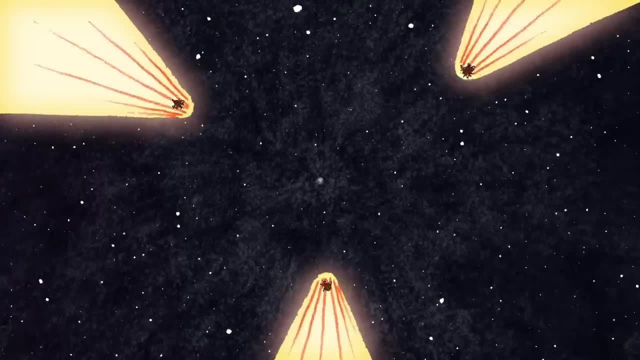 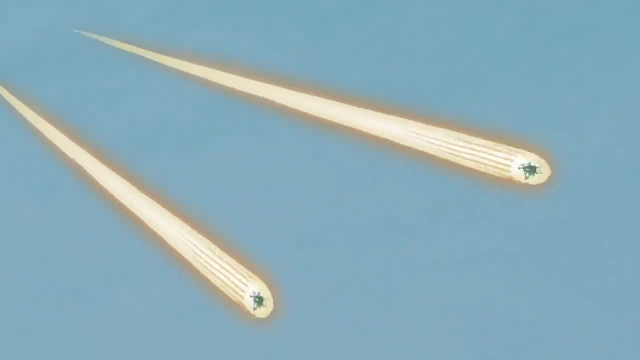 and some of these particles have traveled for billions of years before reaching Earth. When they enter our atmosphere, they collide with the molecules there generating energy. When they enter our atmosphere, they collide with the molecules there generating energy, generating secondary cosmic rays. 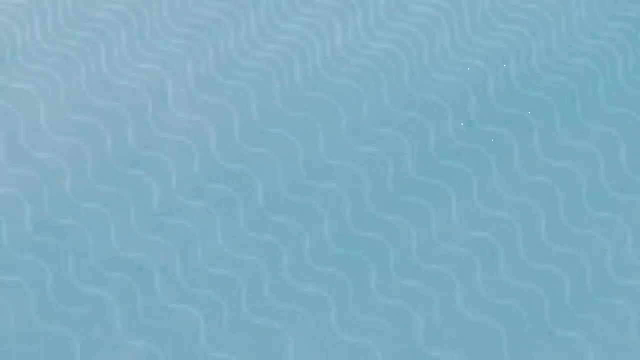 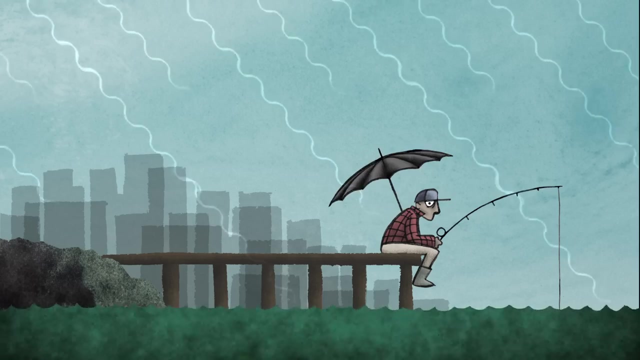 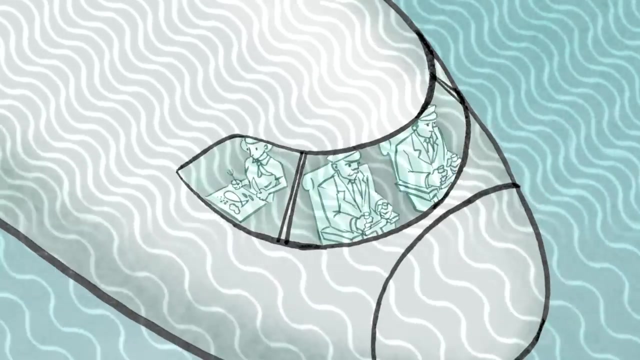 lighter particles with less energy than the original. Most of these are absorbed into the atmosphere, but some are able to reach the ground, even passing through our bodies. At sea level, this radiation is fairly low, but people who spend a lot of time at higher altitudes